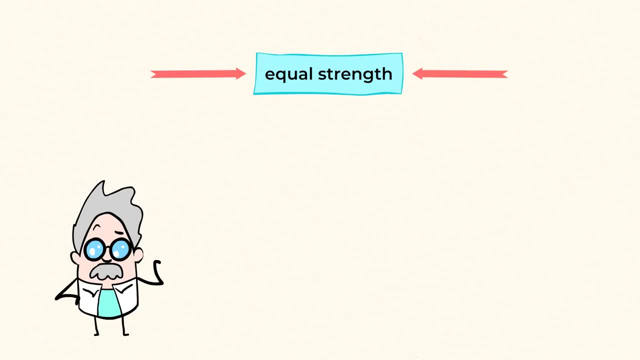 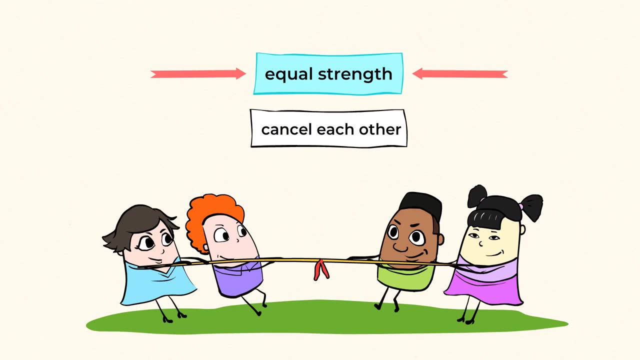 When forces With equal strength and opposite direction combined, they cancel each other. Think of a game of tug-of-war. You know what I'm talking about: When both teams are pulling equally on the rope, even though they are pulling the rope in opposite. 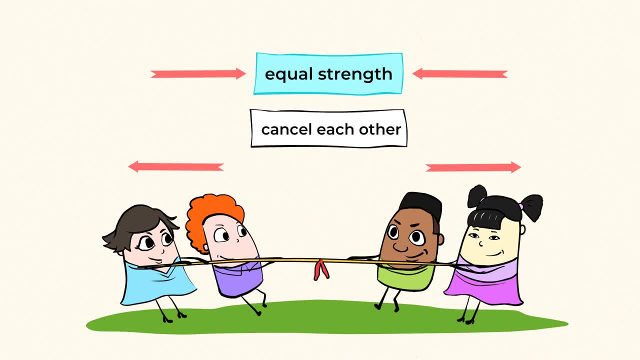 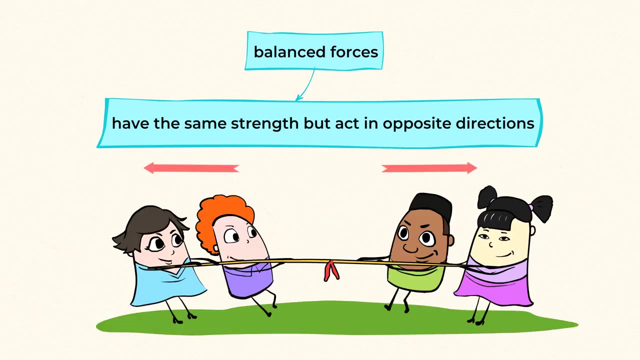 directions. if they both pull with exactly the same amount of strength, they do not cause a change in motion. These forces here are called balanced forces. They have the same strength but they act in opposite directions. Because of that, you'll hear that balanced forces can cancel. 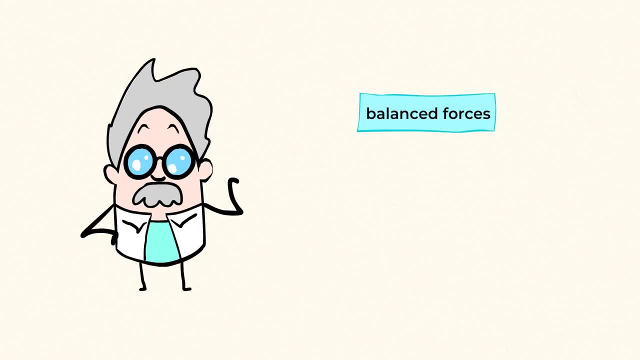 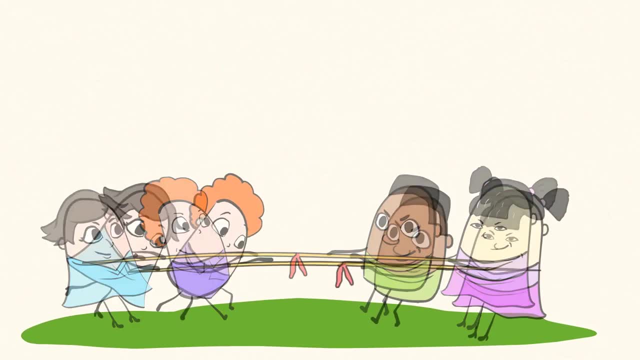 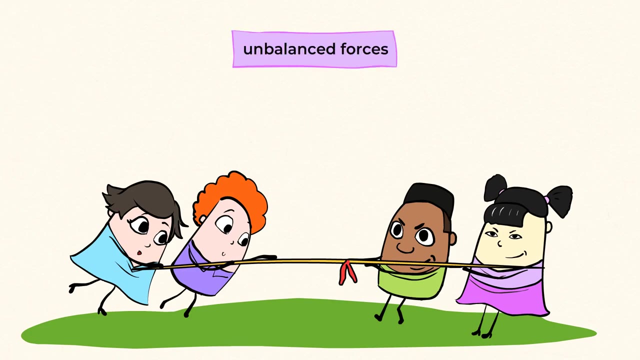 each other out. Now, if there are balanced forces, guess what other forces we may have Unbalanced? exactly Back to our tug-of-war. The moment this flag goes in the direction of one of the teams, the forces applied here become unbalanced. The unbalanced forces have different. 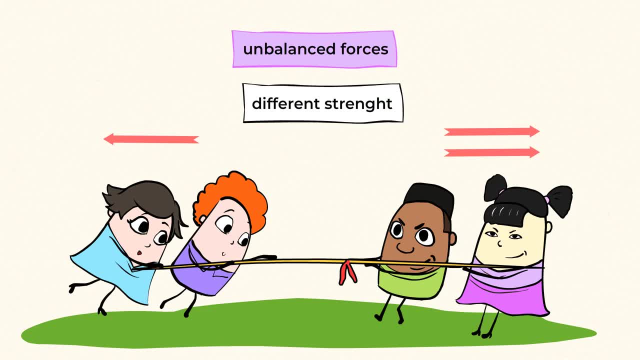 strengths. Because of that, they can cancel each other out. So if there are unbalanced forces, the rope starts moving and one of the teams wins by pulling it towards themselves with greater strength than the other team, Which means that unbalanced forces can cause an object to move. 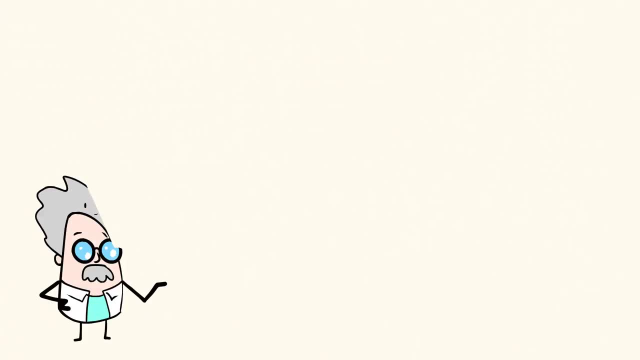 or change its motion. Let's explore another scenario. Say two boys are arm wrestling. Now they're pushing in opposite directions and they're both pushing the same amount, which means they are exerting the same amount of force. We could say that they represent balanced forces. Well, what do you think happens if someone else? 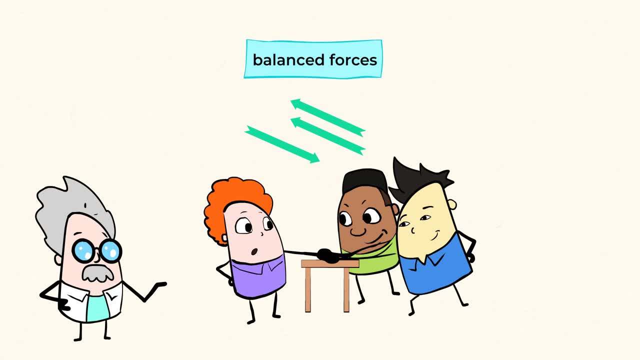 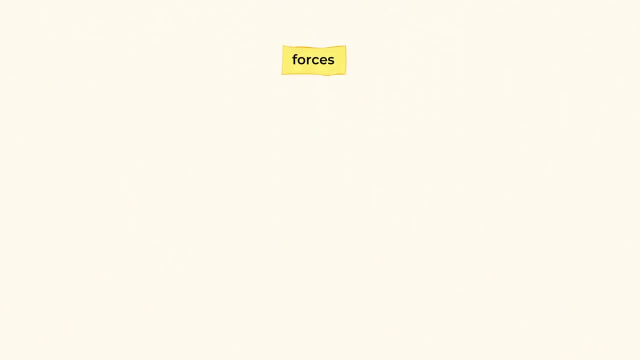 comes to help out one of the boys and they push together. That's right. The forces are now unbalanced And, although it's clearly cheating, the boy who received help will win the arm wrestling contest. Our next task will be to compare and contrast balanced and unbalanced. 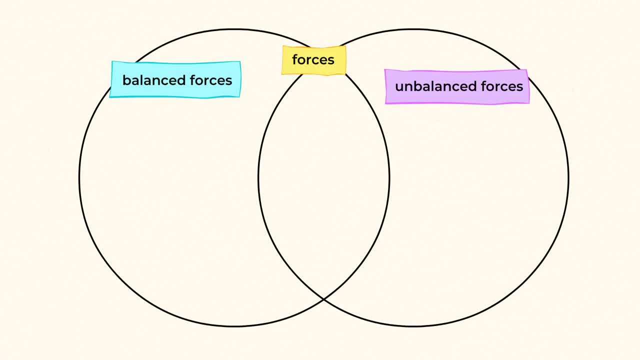 forces, How they're doing and how they're not. So let's start with the unbalanced forces. Here we go. Balanced forces are forces of equal strength and opposite directions. Because of that, the object affected is at rest or not moving- The easiest way to remember it. Think about the.